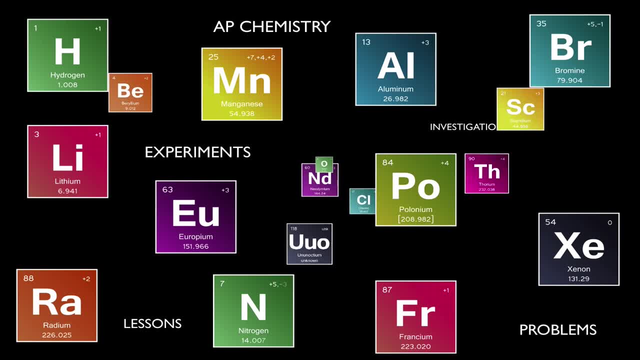 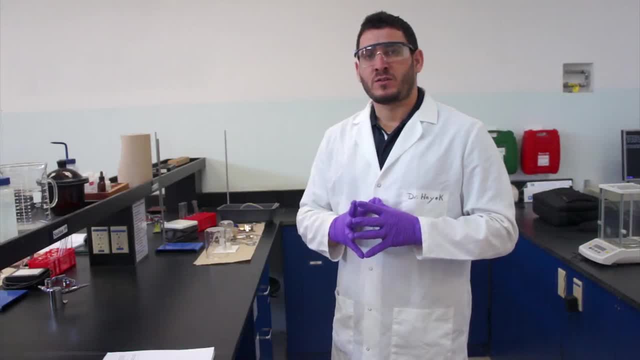 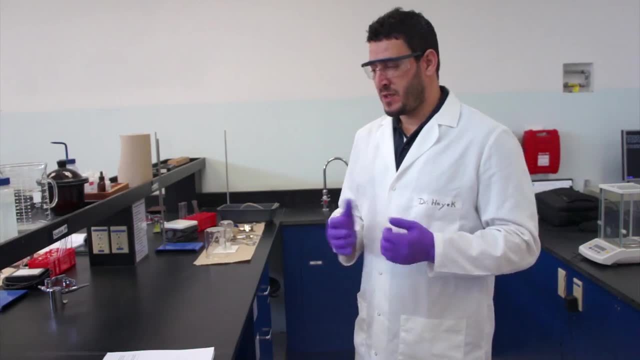 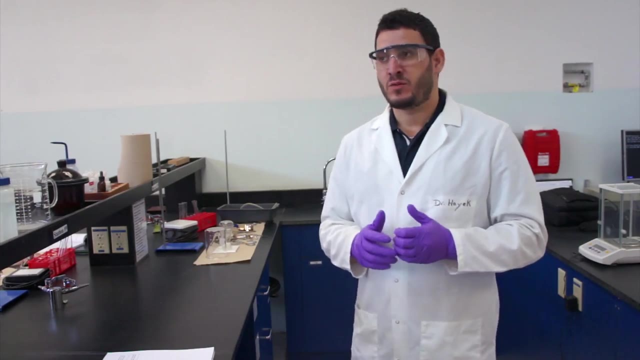 Okay, today's experiment is experiment three. This is type of chemical reactions. We have different types of chemical reactions. We have here one, two, three, four, five different types. We will define each one and we will run an experiment on each one. The first one: 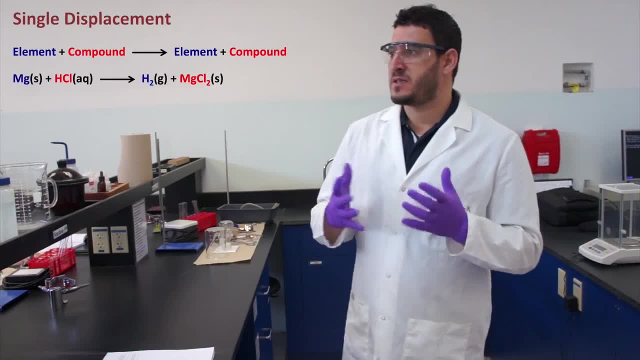 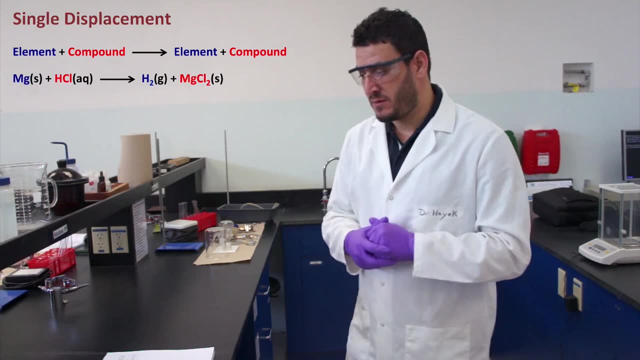 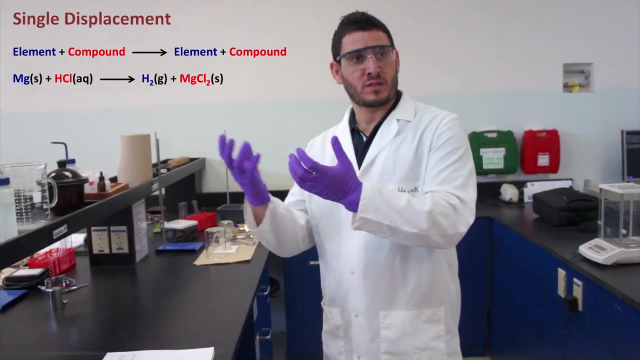 we have is single displacement. Single displacement reaction. this is when one element reacts with a compound to give another element plus compound. Okay so, element plus compound. they give element plus compound For the single displacement. this is when, for example, 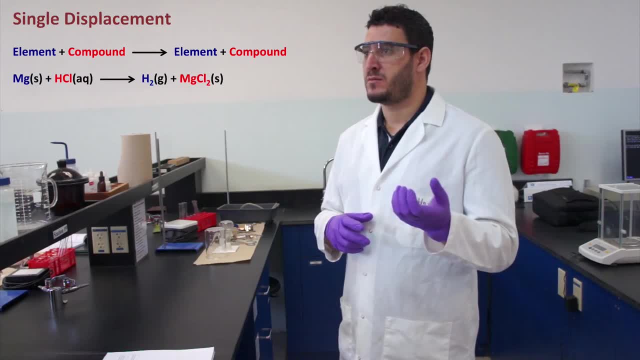 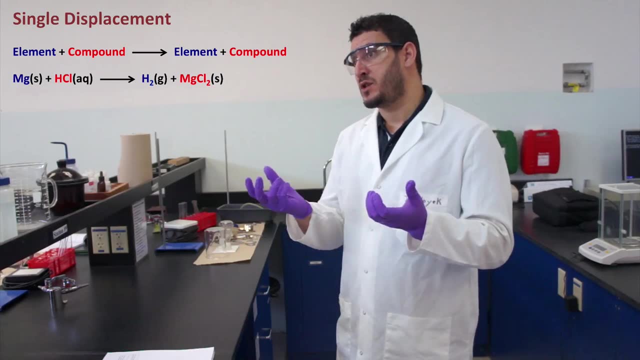 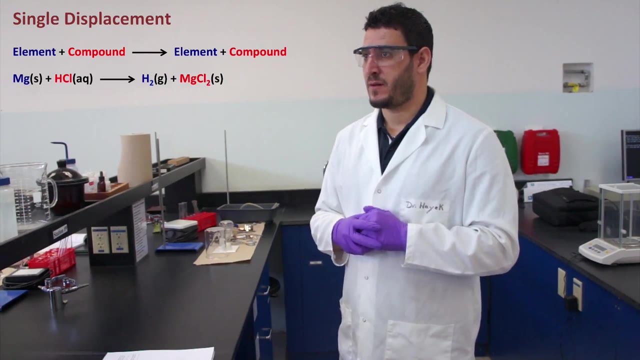 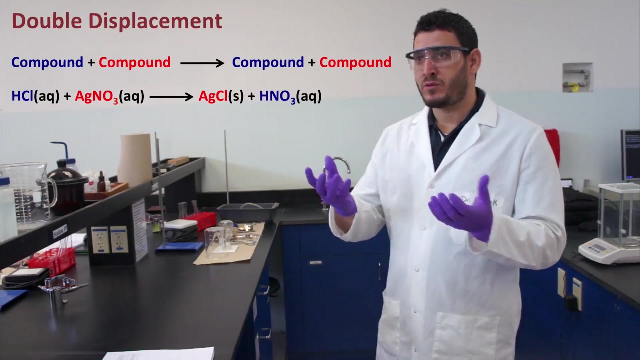 an element such zinc or magnesium reacts with a compound like HCl To form an element, which is hydrogen gas, plus magnesium chloride, which is a compound. Okay, now for the double displacement. this is when you have a compound plus a compound. 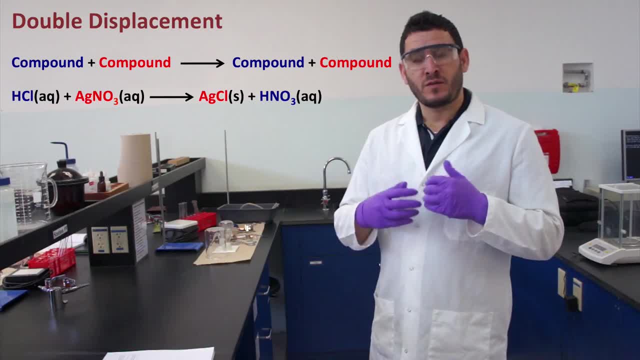 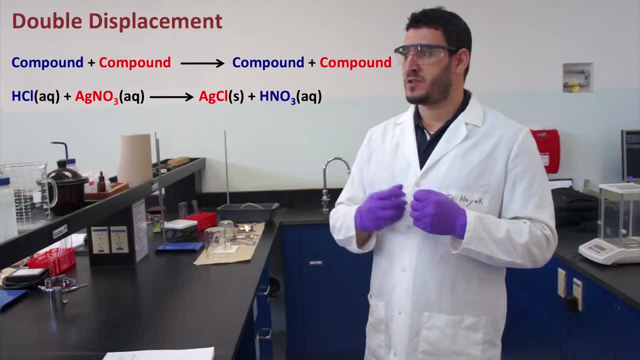 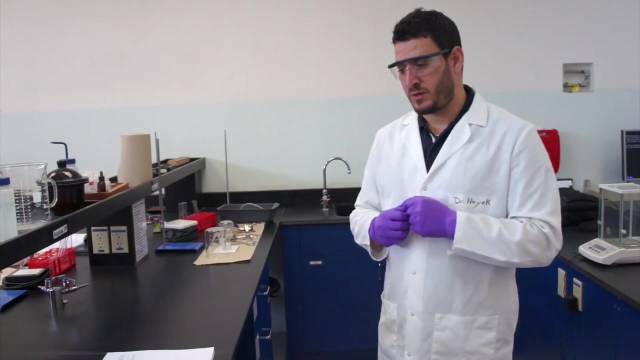 to give you two other compounds. For example, if you mix HCl plus silver nitrate, AgNO3,, that's going to give you AgCl plus HNO3.. Okay, which is nitric acid. So compound plus compound gives you compound plus compound. Decomposition reaction. decomposition reaction from its 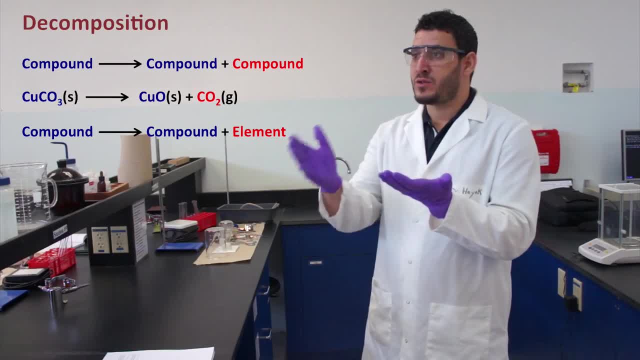 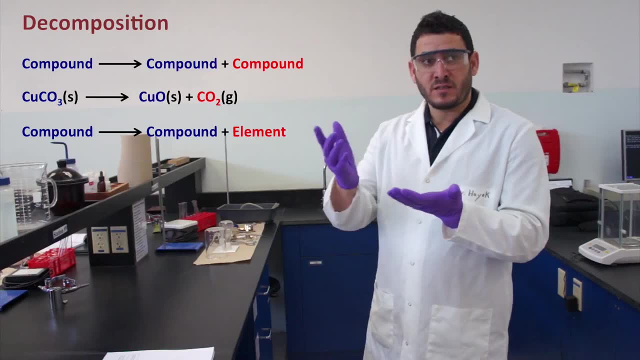 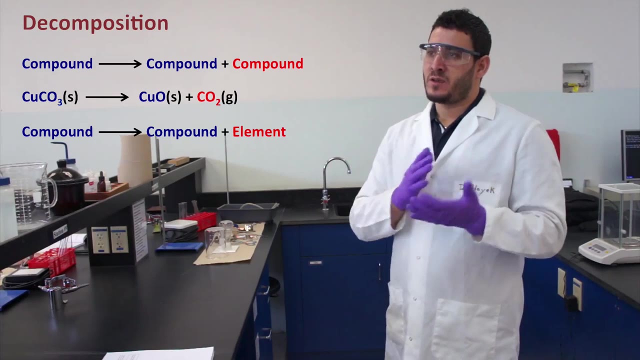 name. this is when you have a compound and you break it into an element and a compound, or two compounds- Okay, reactants, it's only one compound that you will break it down. so an example to decomposition reaction is like when you have copper carbonate- CuCO3- you will. 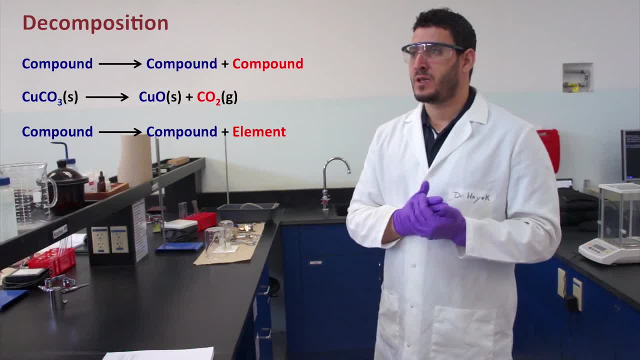 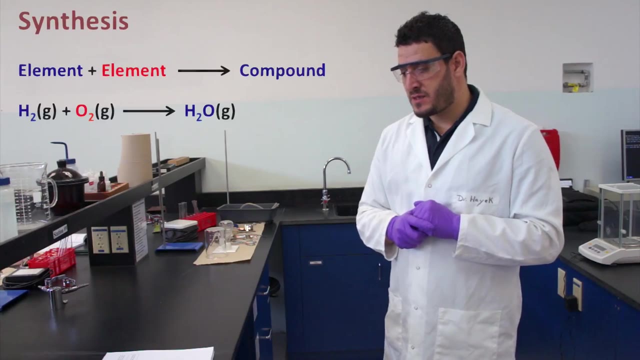 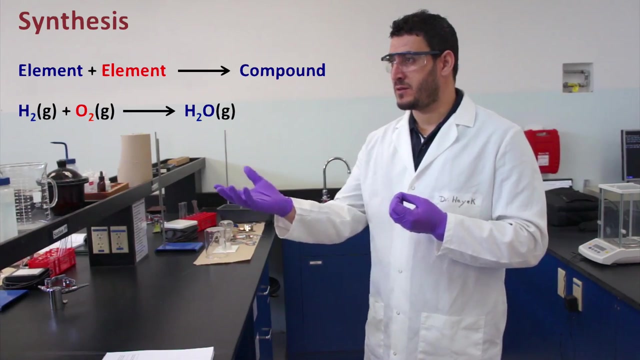 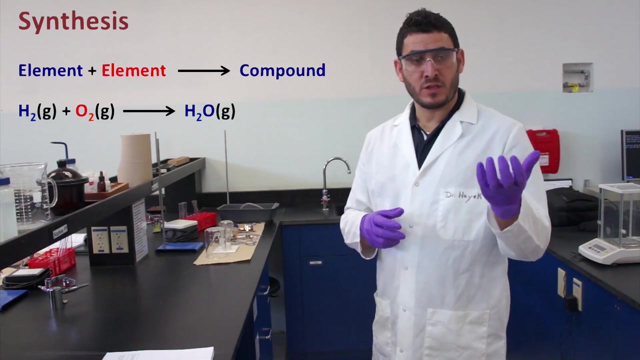 heat it up and you break it into copper oxide, CuO, copper oxide plus CO2. another type of chemical reactions is synthesis. synthesis: this is when we react two elements together or two compounds together to give you a compound. an example to synthesis reaction now, if you combine hydrogen, 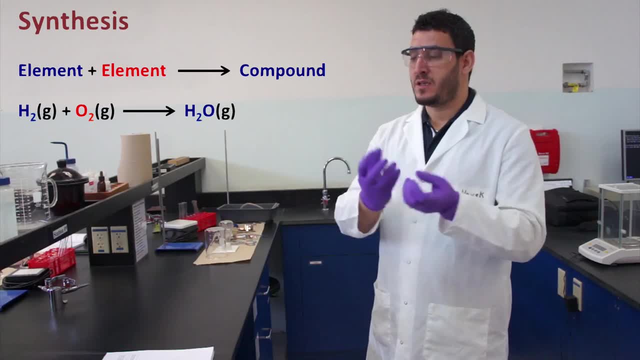 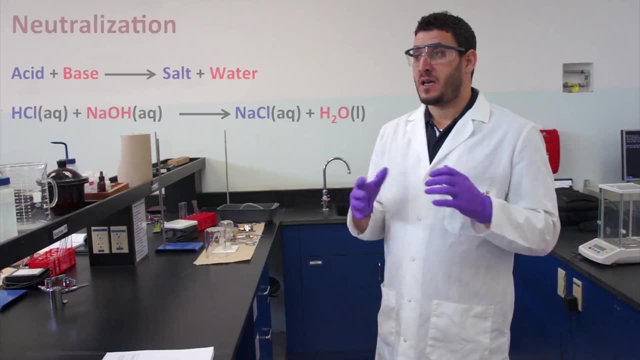 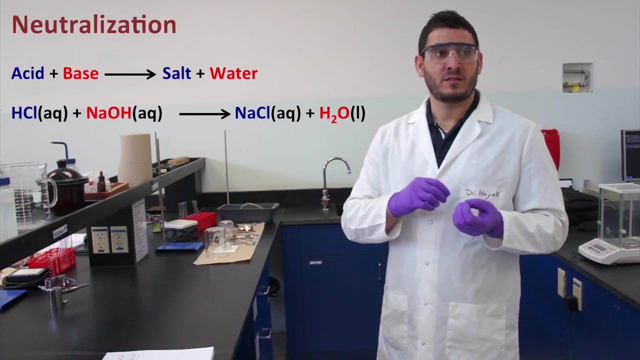 which is an element, plus oxygen, which is also an element. they will give you water, which is a compound. this would be the simplest reaction that we will do today, and the last one is neutralization. neutralization: usually this is the reaction between acid and base. okay, so that's the reaction between acid and 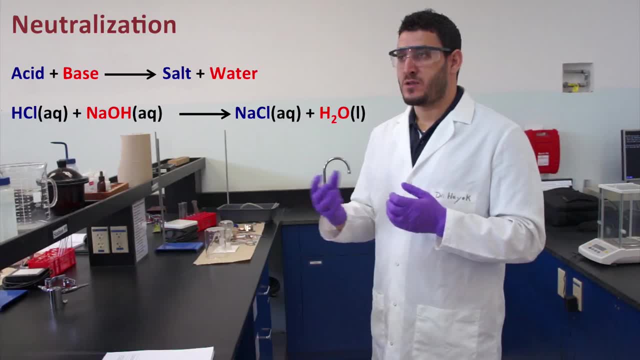 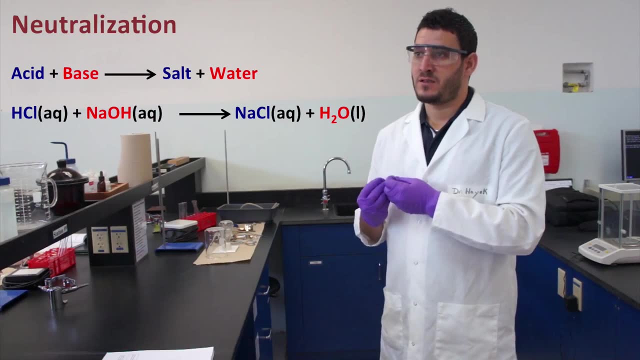 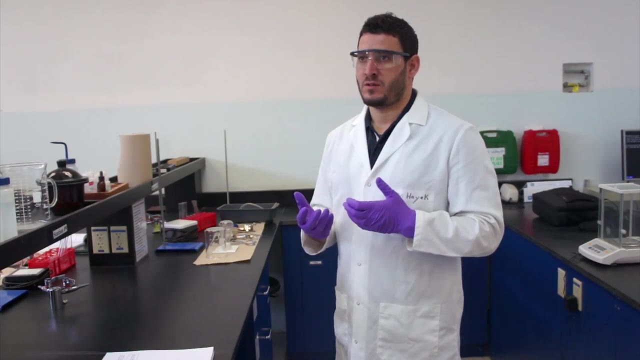 base to give you salt plus water. so, for example, if you have HCl plus NaOH, sodium hydroxide will give you the NaCl, the salt plus water, which is the H2O. so now we will be doing an experiment on each type of chemical reaction. the first one we will do the synthesis reaction. okay, 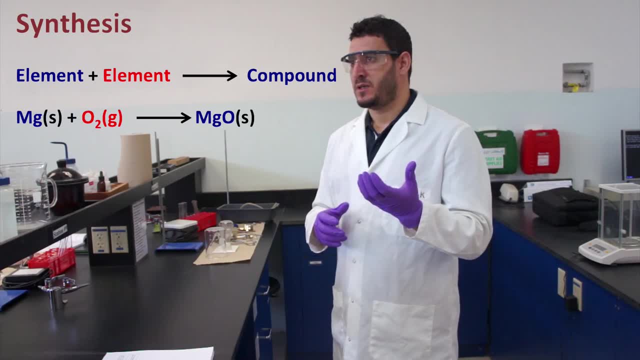 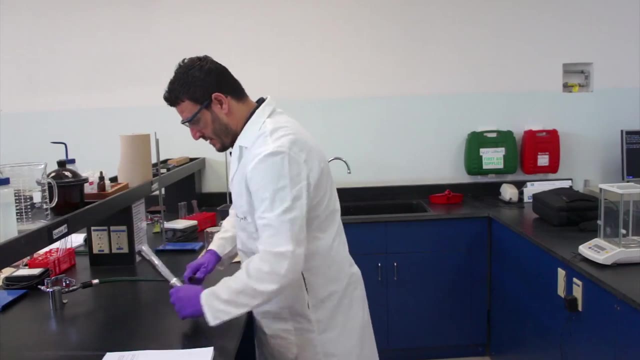 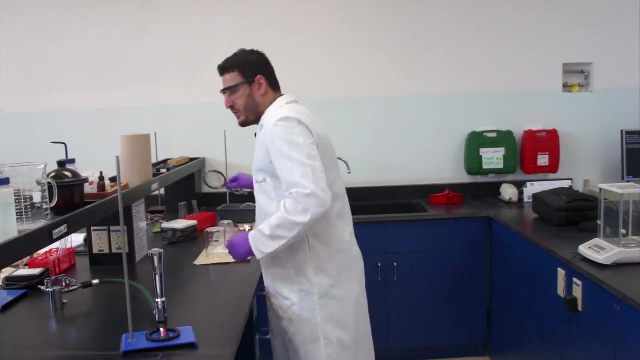 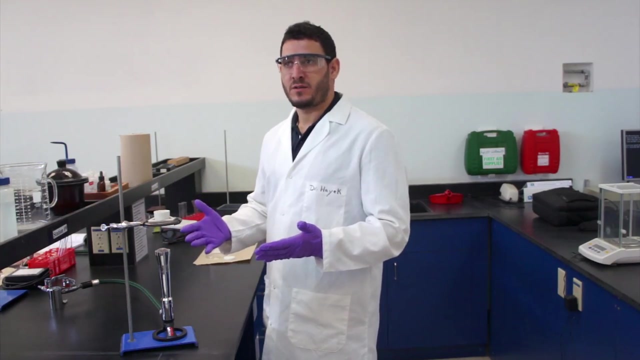 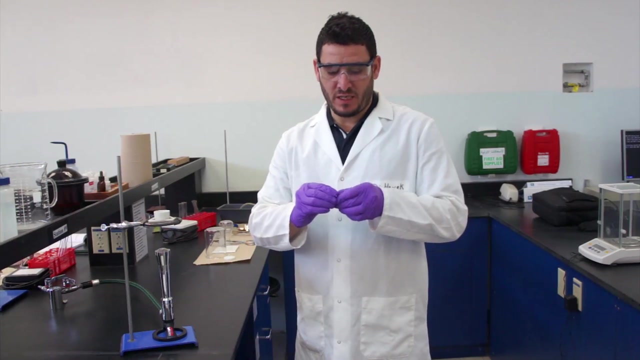 now we will have magnesium ribbon. we will heat it up to react with the oxygen to give you magnesium oxide. so the reaction set up. I will do it quickly, you right? so this is your experiment 3 setup. so your magnesium. you will just roll it like this. okay, so you just make it small. 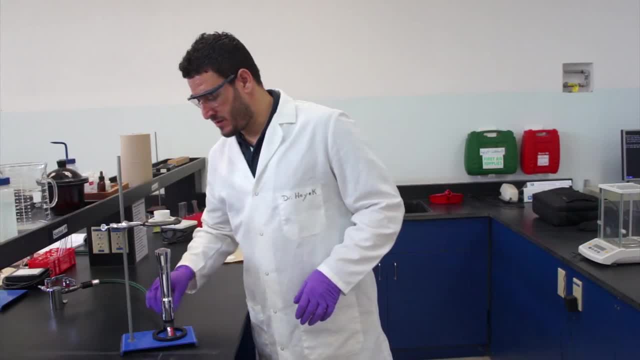 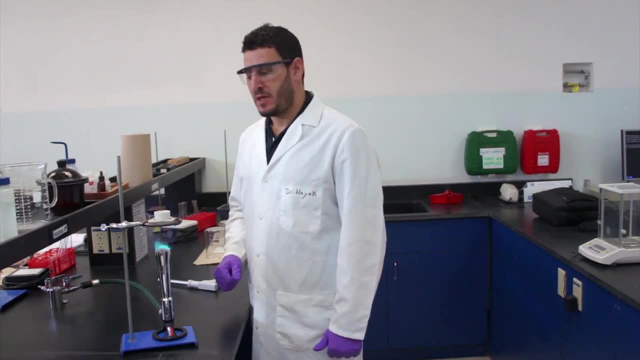 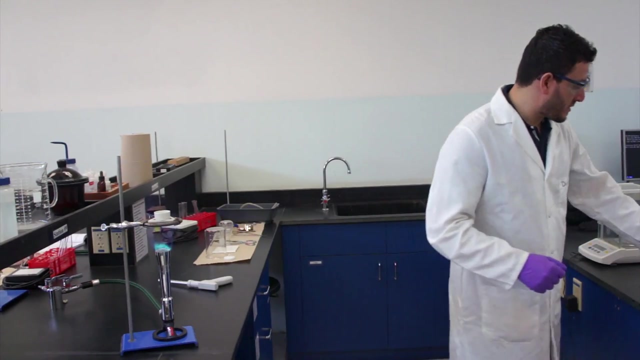 like this and just put it in your gr Virgin. you will start your pontoon burner and you will just heat it up to react with the" research hypot stereotype: wait and look what is happening inside your crystal, basically, what is going to happen inside your crystal. 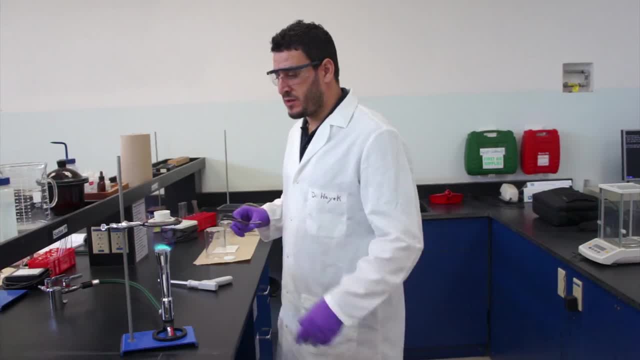 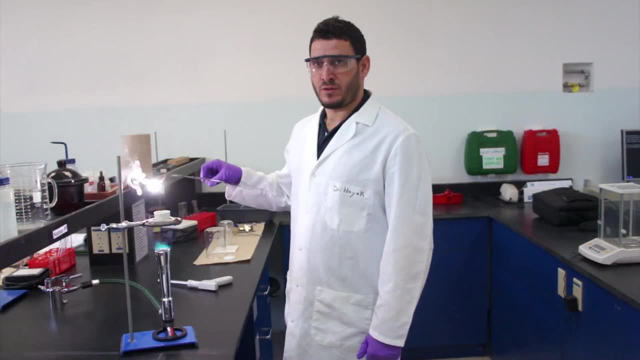 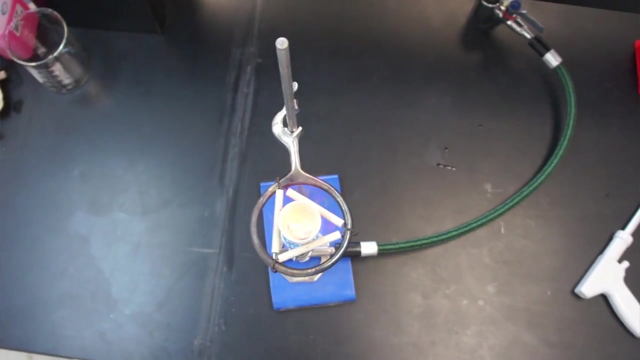 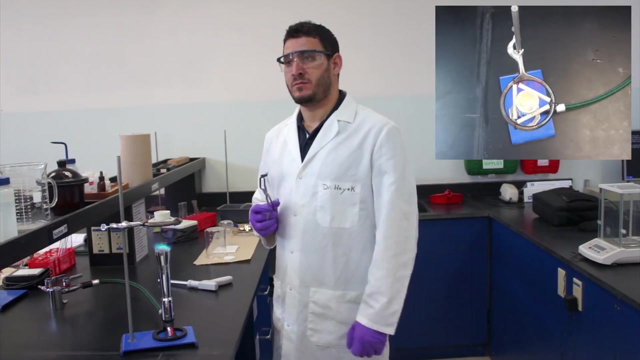 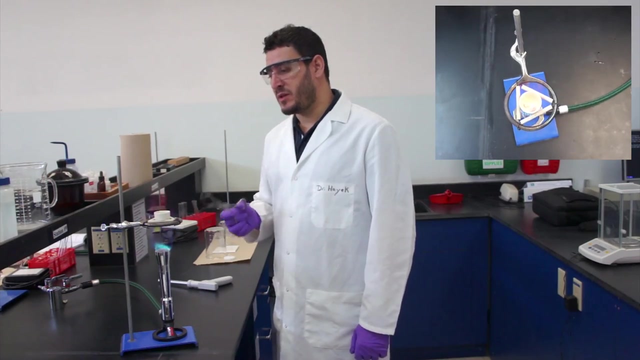 I will show to you now. so do not look directly to the flame, okay, because this is going to be strong. so you can see basically what we are doing here. we are burning the magnesium strip to form. look at the ash for magnesium oxide. now this will happen inside your crystal when the crystal 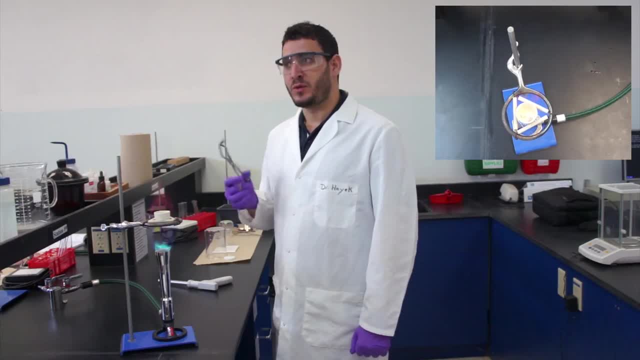 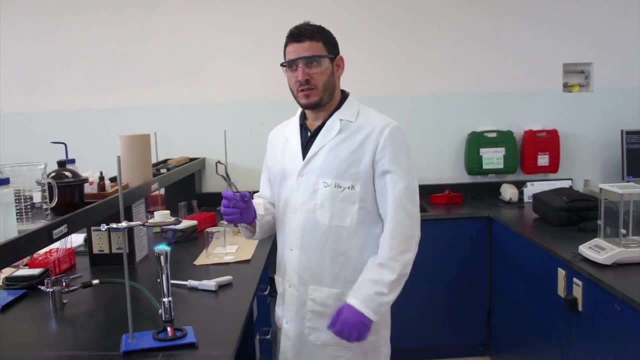 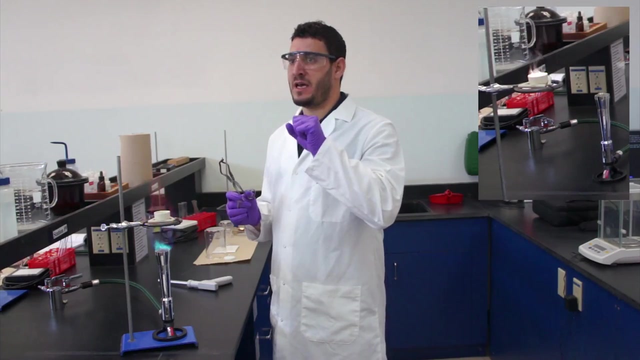 gets too hot, the magnesium strip will burn inside, which means will react with oxygen to give the magnesium oxide. now when to stop your reaction. this is when you see the glowing of the magnesium strip. this is when the reaction starts and when the glowing ends, this is when your reaction ends, so you can turn off the ponser burn. 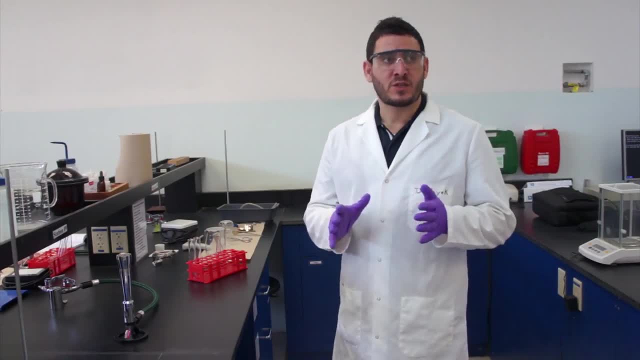 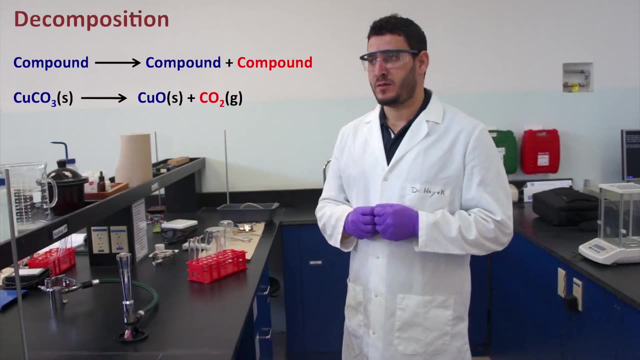 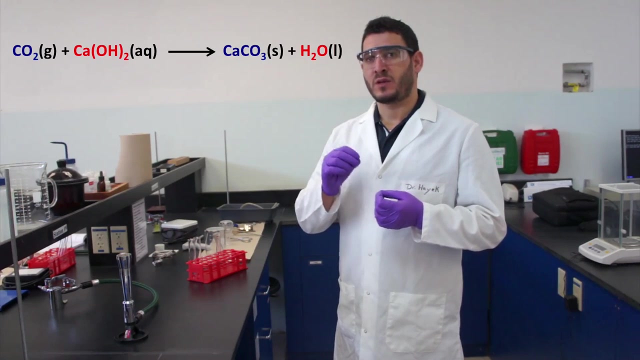 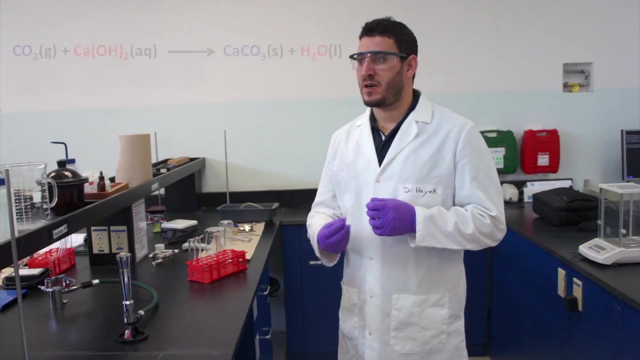 so now the next experiment is the decomposition reaction. this is when we will heat copper carbonate to give copper oxide plus carbon dioxide to detect the carbon dioxide from the magnesium and the magnesium, and you can see that the Carbon dioxide is known to react with calcium hydroxide, CaOH2, and it will give the calcium carbonate which will precipitate out of the reaction. 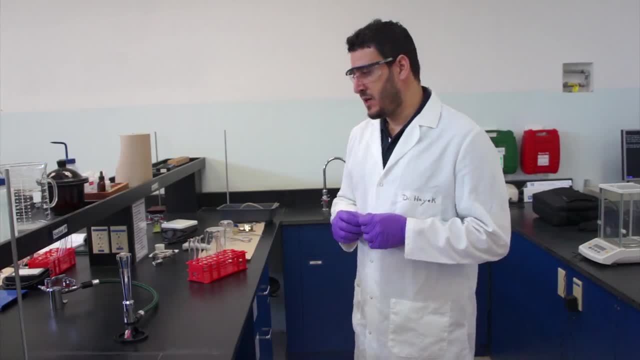 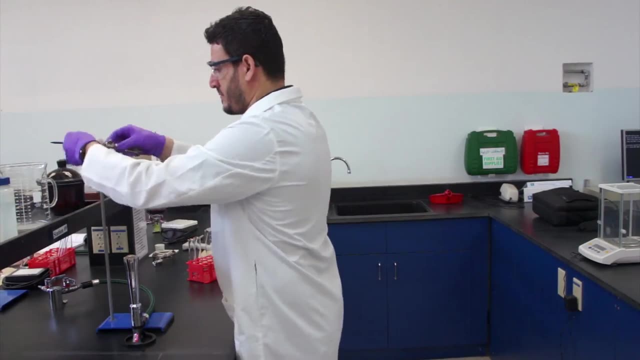 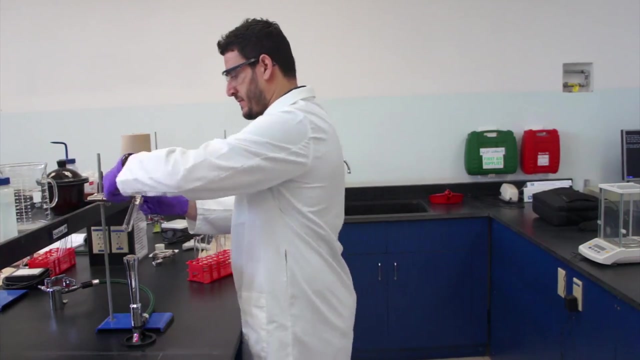 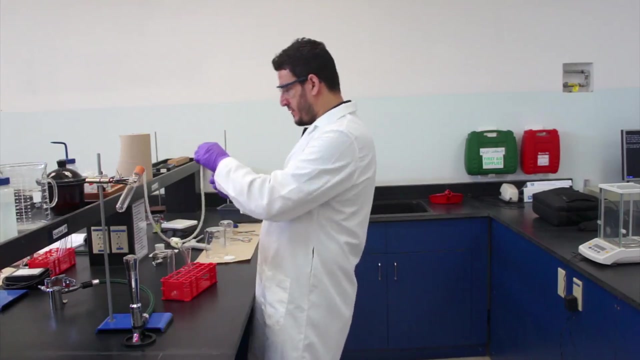 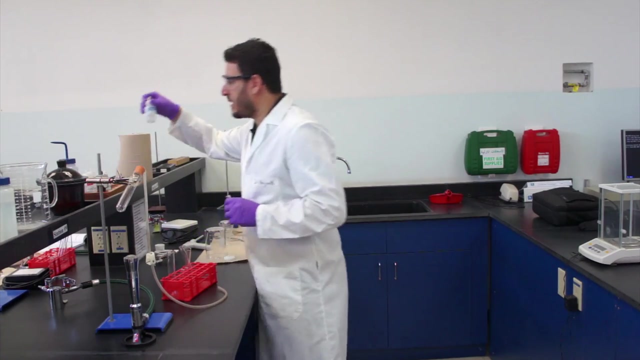 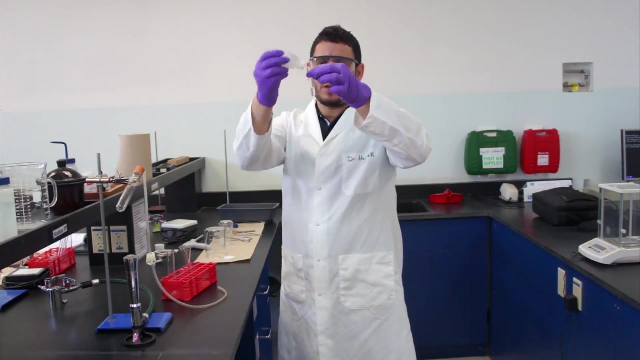 So we will see a white precipitation. Now to do this reaction, the experimental setup is the following: You will take calcium, calcium hydroxide, Now to the small tube, we add calcium hydroxide. We don't add much because we still need room for the pipe. 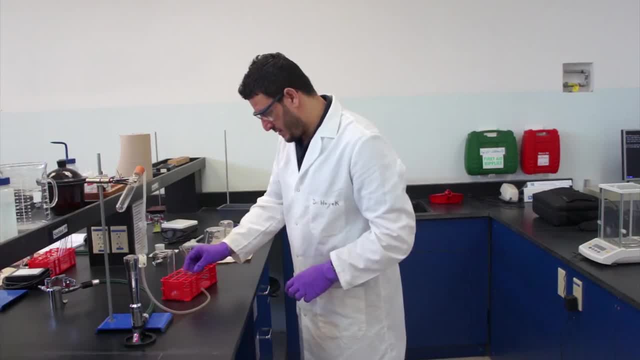 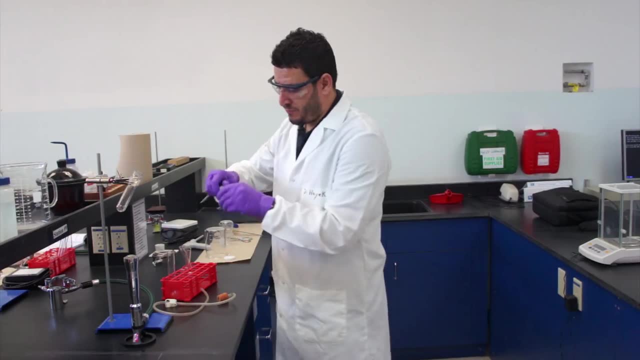 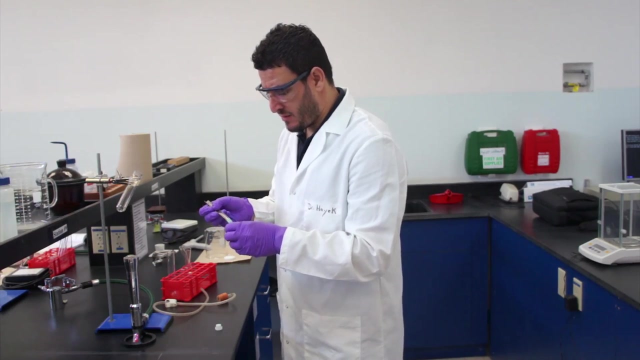 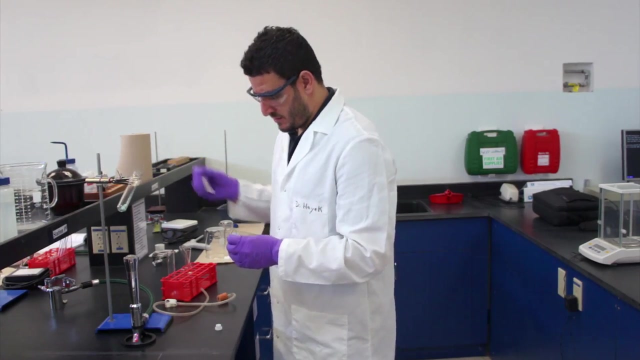 So we'll leave it here Now, inside this tube. we will add enough amount. Now your lab manual tells you how many grams you should take. I'll add this much. That's enough for my reaction. Make sure that it goes to the bottom of my tube. 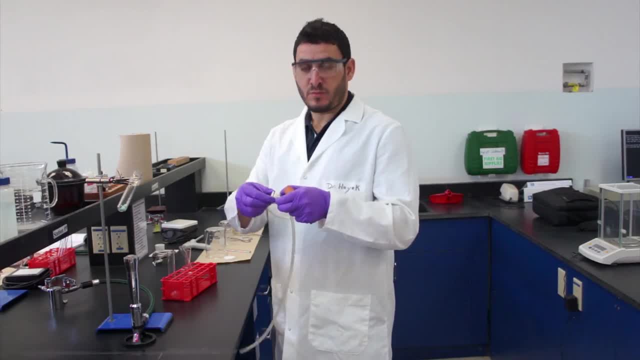 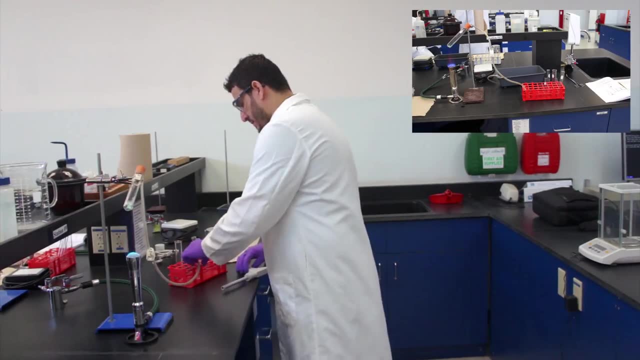 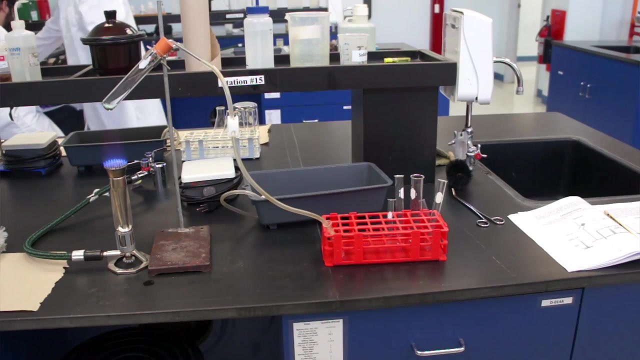 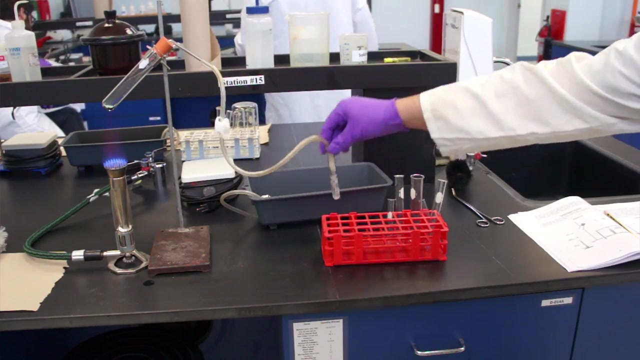 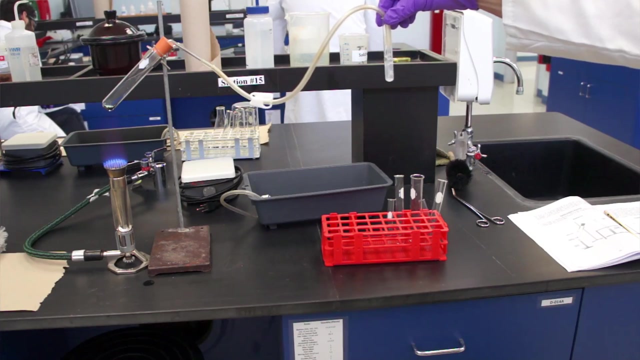 And now I'm ready to start my reaction. Now, before you start your reaction, make sure that you have the right amount of calcium hydroxide. Make sure that the pitch clamp is open. You can watch what's happening here. As long as you see gas bubbles coming, it means your reaction is working. 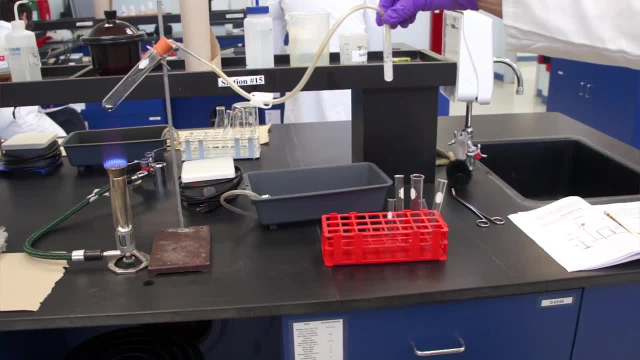 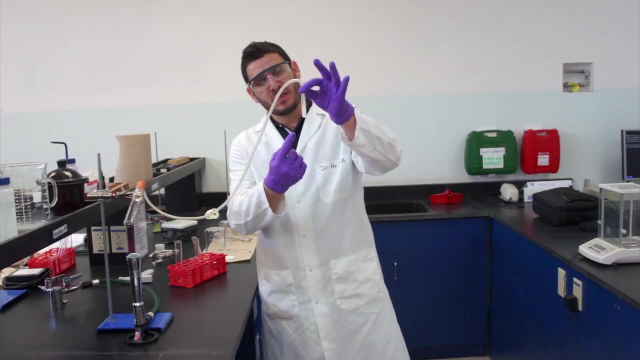 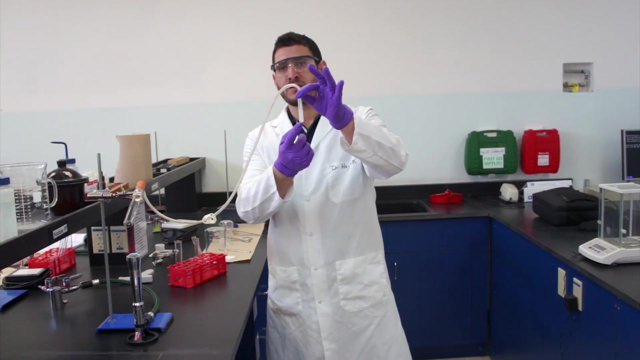 See, we're having more and more of the gas bubbles. So if you look closely to the solution, you can see that it's becoming cloudy. Okay, So what is happening here? you have the carbon dioxide coming here, reacting with the calcium hydroxide to give calcium carbonate. 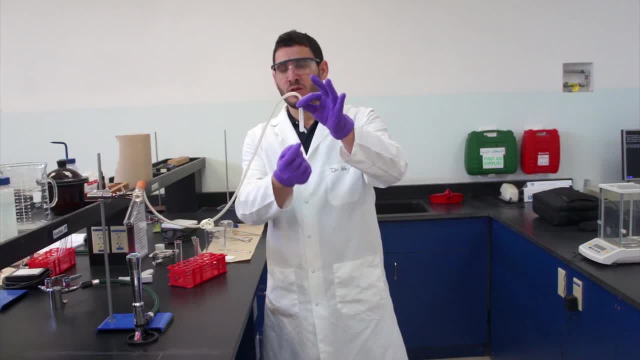 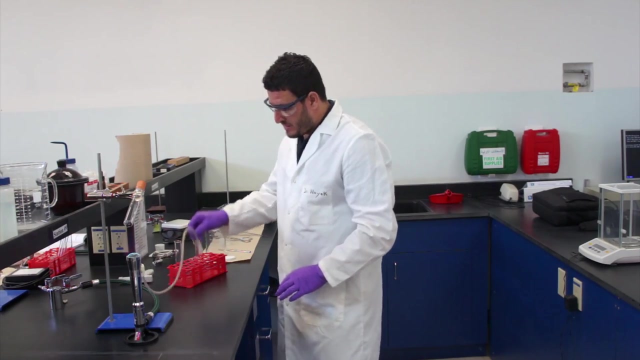 which is not soluble in water, and it will precipitate. Now the reaction between carbon dioxide and calcium hydroxide is considered as a synthesis reaction. So when do we stop this experiment? It's either when we see enough white precipitating here. 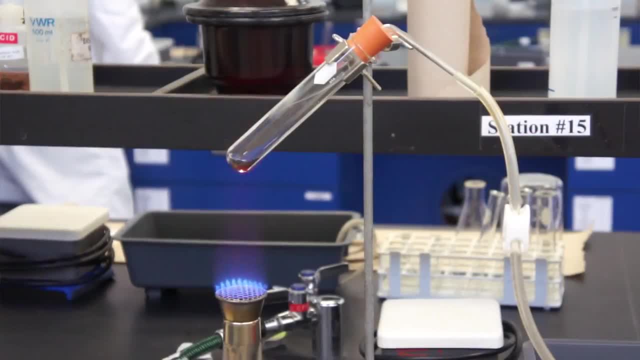 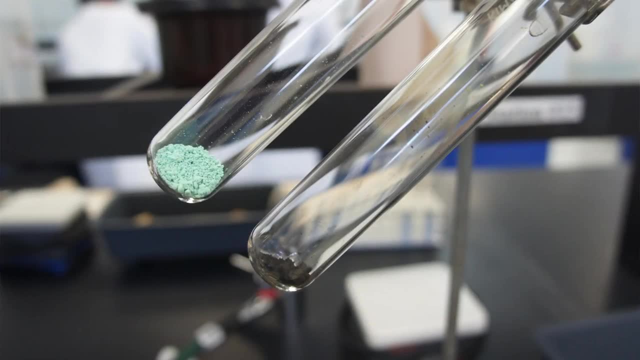 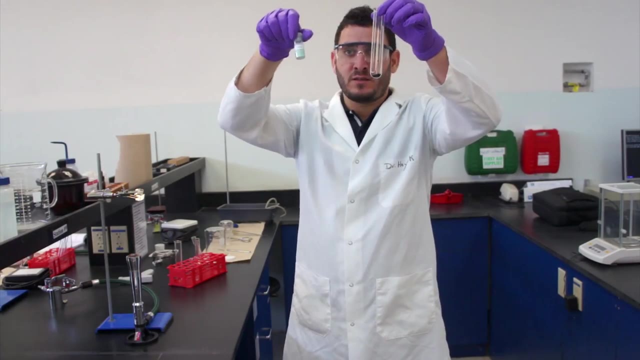 or we don't see any bubbles coming out. Look at the remaining solid inside your tube. It's a black solid Right, It used to be green solid like this one. Now it's black. This is the copper carbonate, and the remaining solid is the copper oxide. 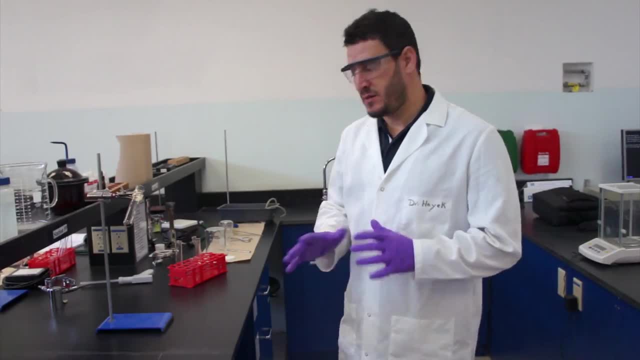 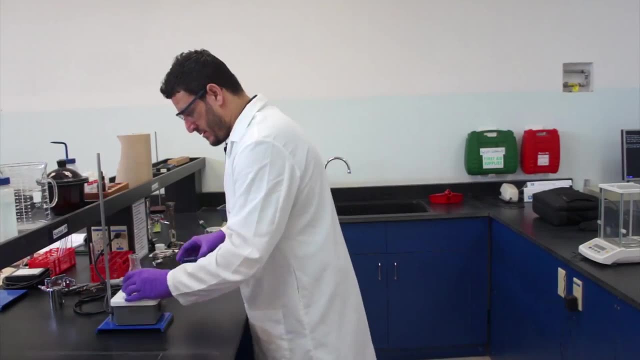 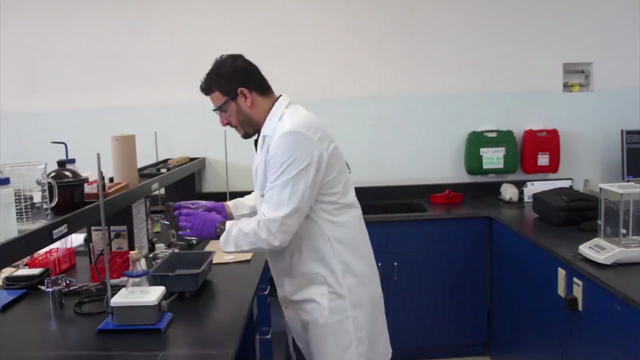 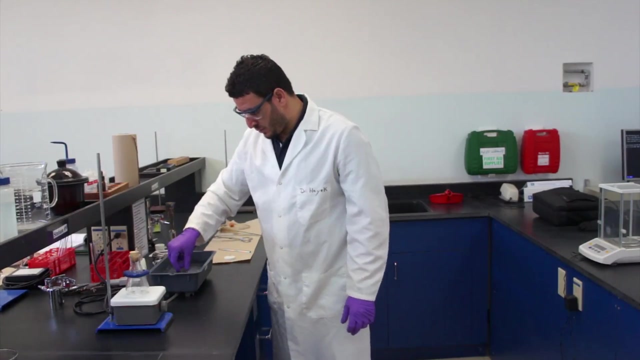 Now for the third experiment. the setup is the following: We're going to fill this one with water. Just put it like this and incline it and let it go. It will all be filled with water. Now you will locate the opening. 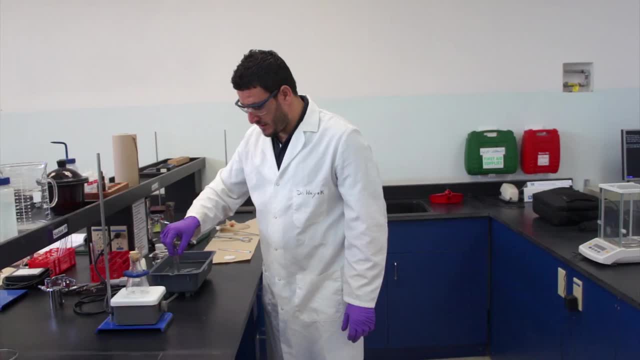 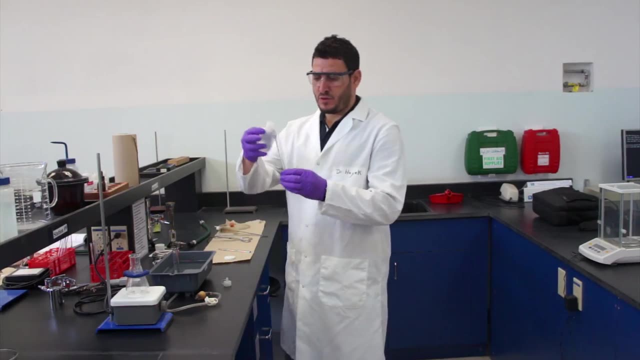 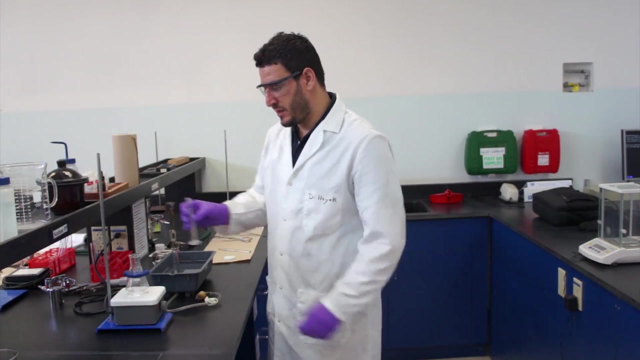 and you just put it in the middle of the opening. So we will need 10 milliliters of the hydrochloric acid- 2 molar hydrochloric acid. You add the hydrochloric acid to your Erlenmeyer. 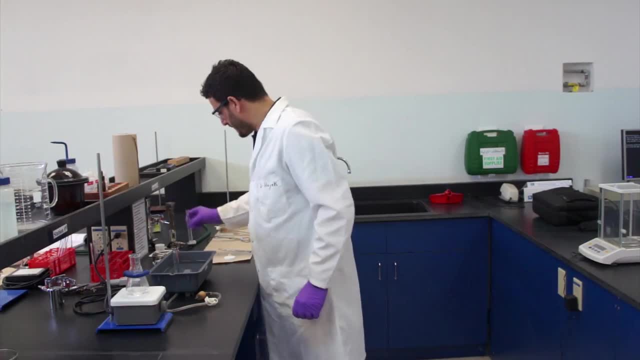 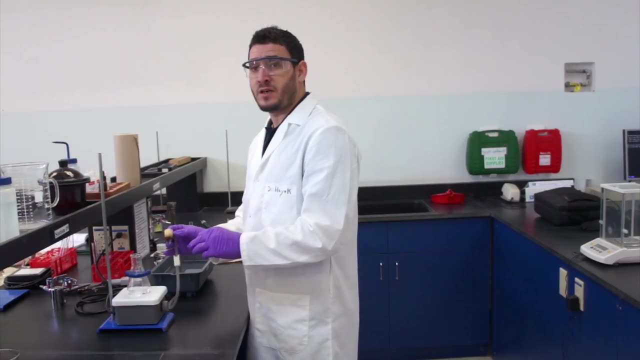 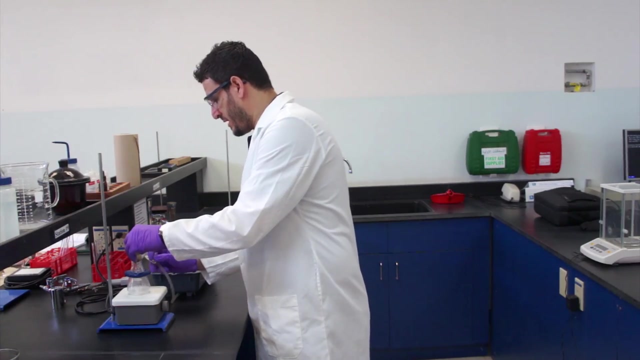 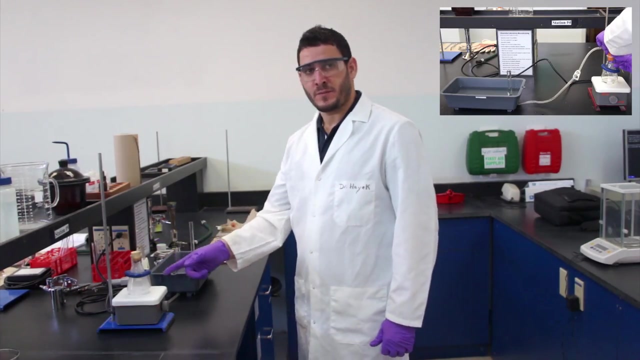 You start stirring. Okay, so now you will be adding your magnesium, closing your container- Erlenmeyer container- and opening the pinch clamp. Look, Open the pinch clamp. There you go, So you can see that the hydrogen gas forming. 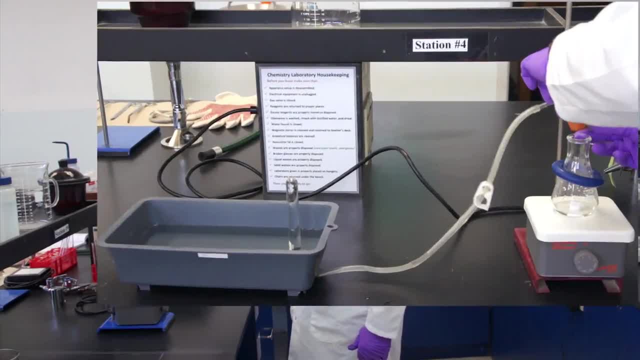 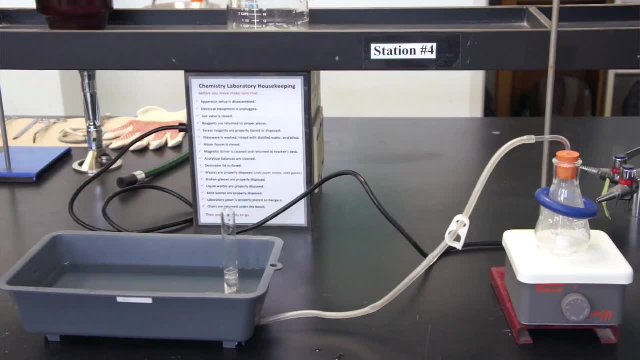 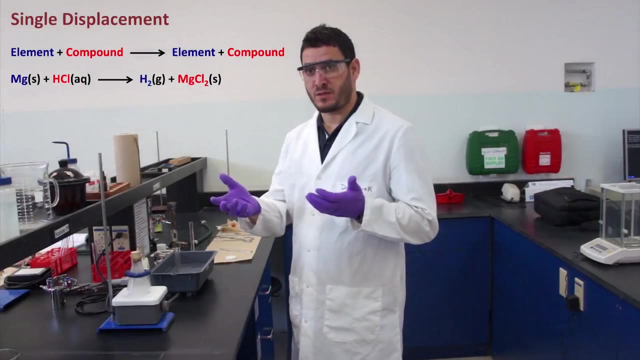 it will come out of the flask and fill in your tube. So, now that the tube is filled with hydrogen, this reaction is a single displacement reaction because you have magnesium, which is an element, plus HCl, which is a compound. It's giving you an element, which is the hydrogen. 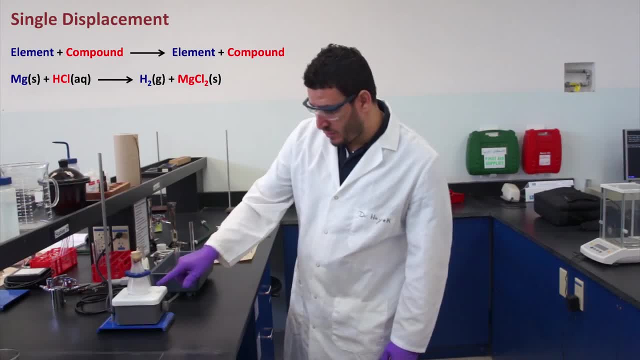 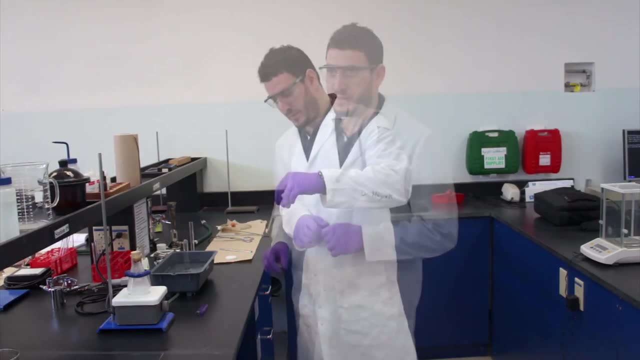 that we collected here in the tube, plus the magnesium chloride that will stay here in the Erlenmeyer Plus. Now to test for hydrogen, we will do the pop sound experiment, We will come with the flame and we will close the tube. 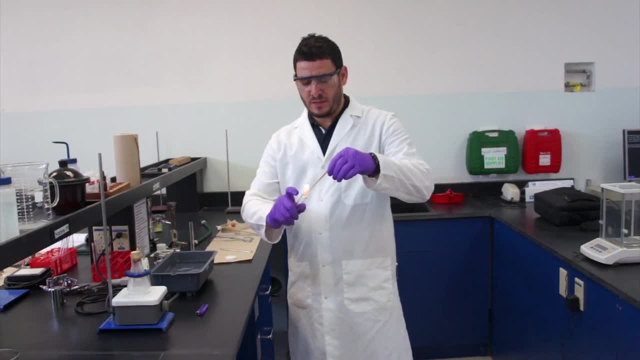 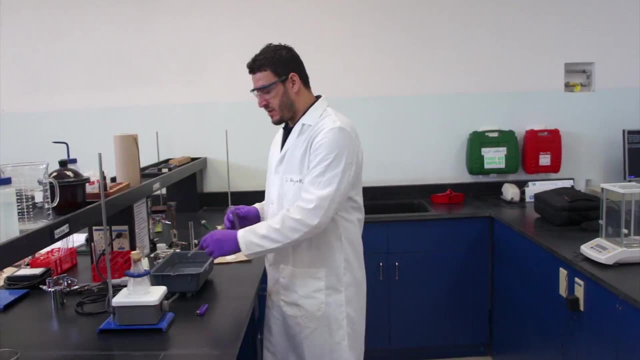 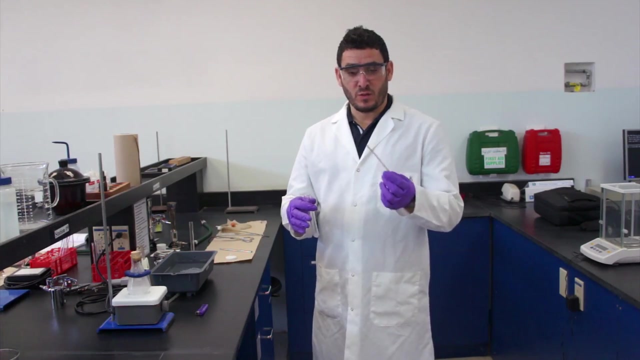 the tube underwater like this and quickly insert the flame inside the tube. Now the hydrogen that's trying to escape the tube is very flammable gas, so it will just react with the oxygen. when you give it this energy, It will react with the oxygen. 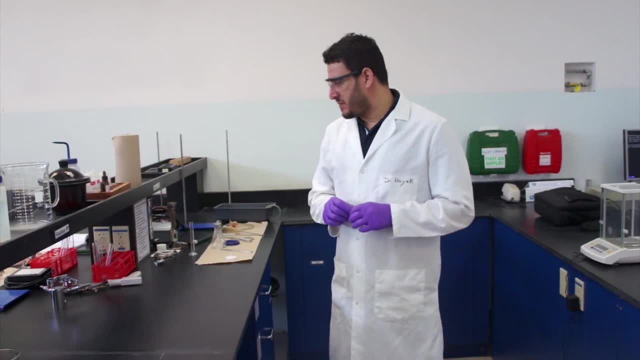 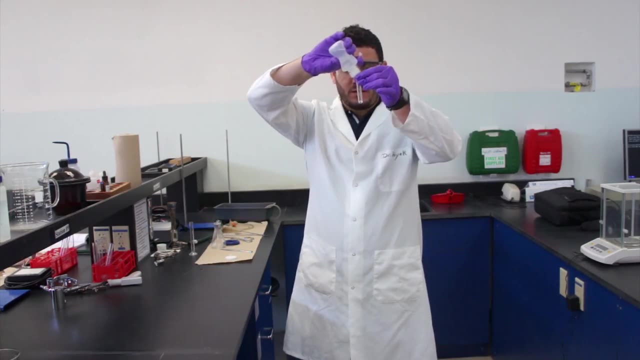 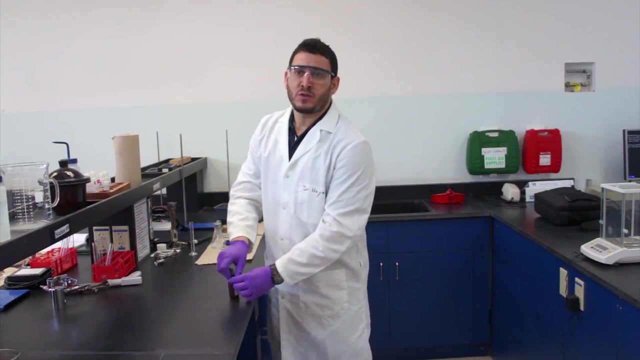 to form water. Now experiment five is a double displacement reaction. We will take hydrochloric acid around two milliliters. Now we said double displacement reaction is a reaction between two compounds. So HCl is a compound and we'll add to it silver nitrate. 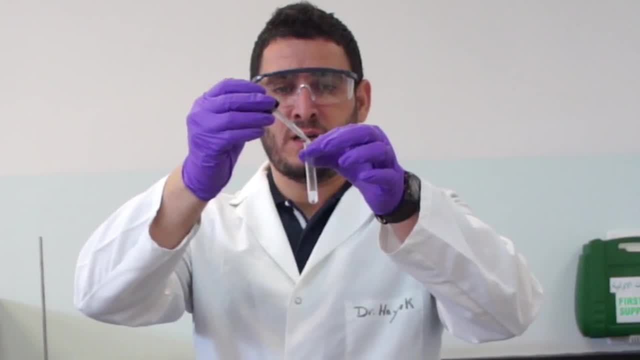 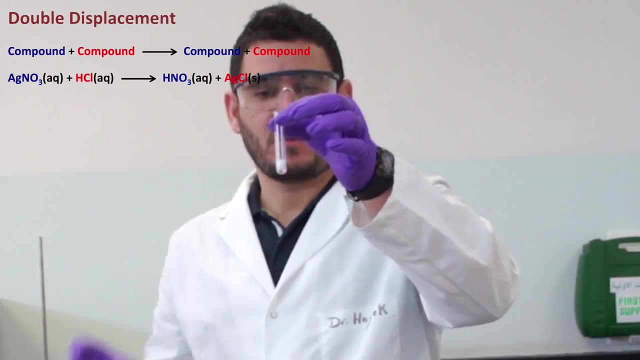 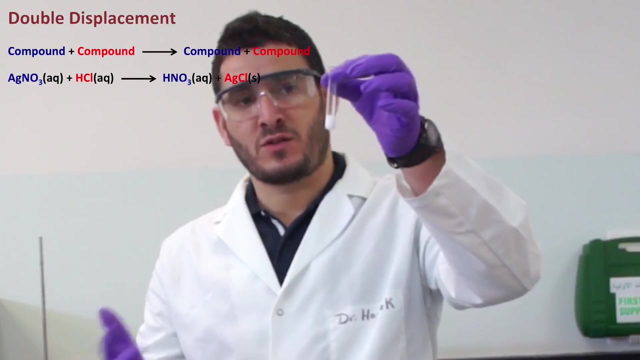 which is also a compound. Okay, Now, as you can see, when silver nitrate is added, it will form a precipitate. The precipitate is silver chloride plus HNO3,, which is a strong acid that will remain dissociated in the solution. 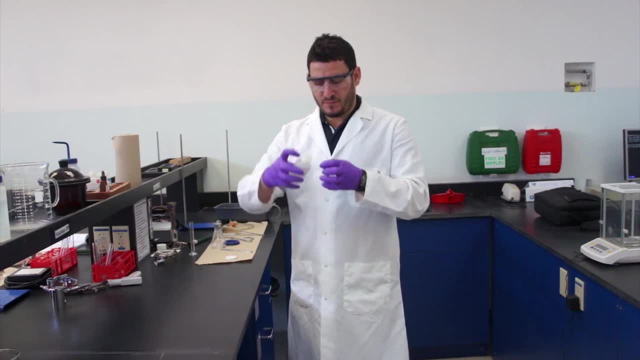 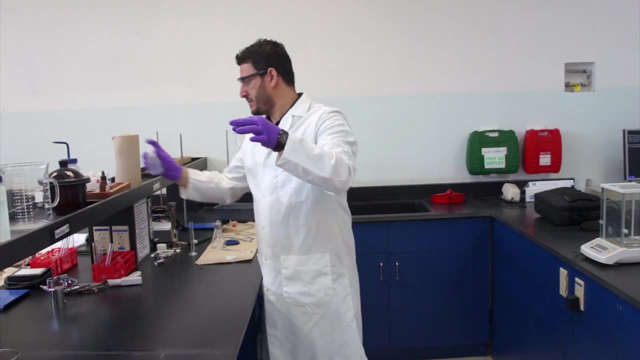 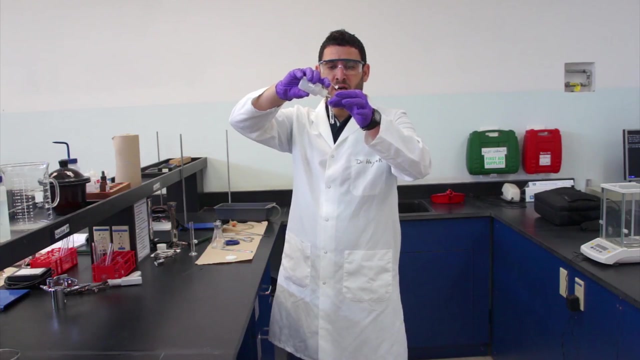 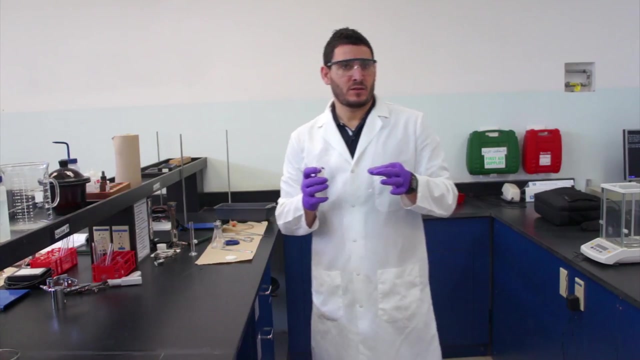 Our experiment six: we will take hydrochloric acid. we will add to it the acid base indicator, the phenolphthalein, we'll add two to three drops And then we will be adding sodium hydroxide. So this is a neutralization reaction.